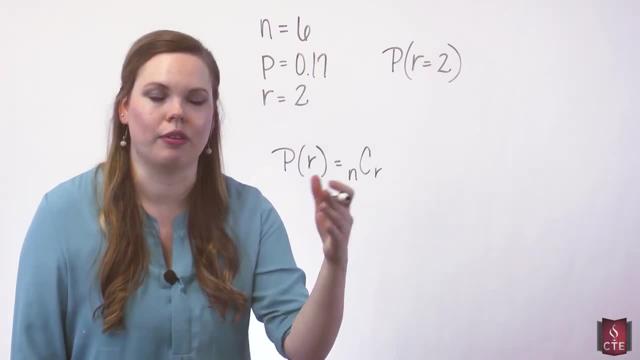 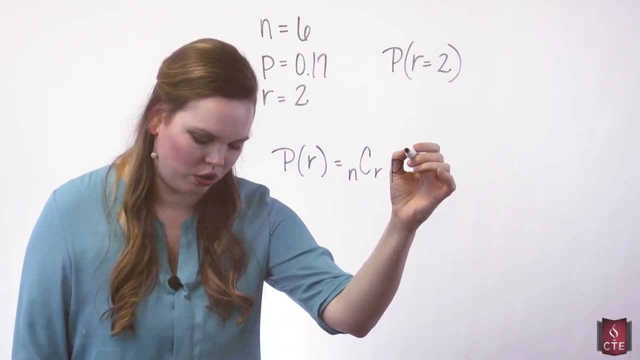 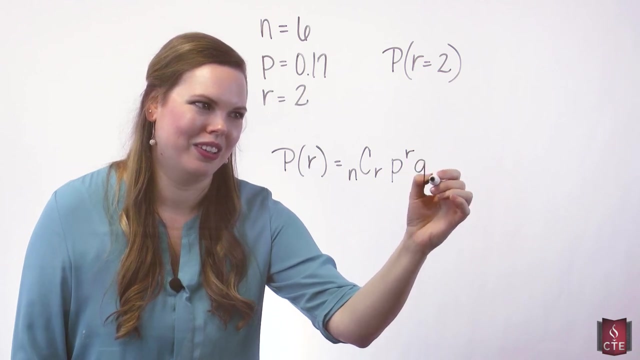 all the different ways that you can select: n objects from… r objects from n. and then we have the probability of a success, p, raised to the number of successes that we want, which is r. And then we have …. have Q raised to the n minus r, which will be the number of failures that we want: Q. 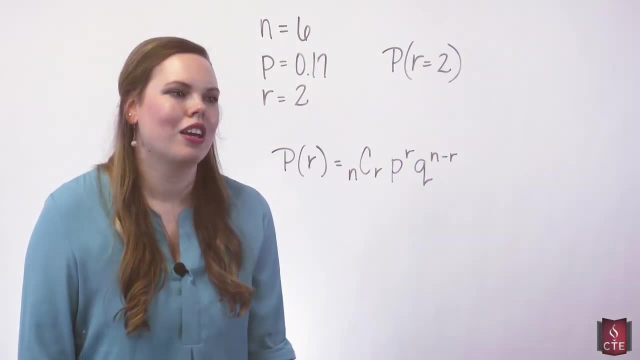 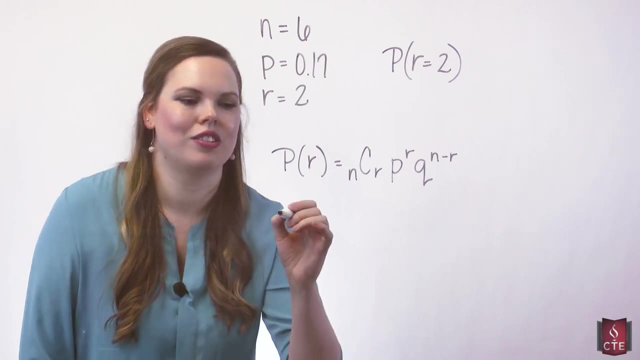 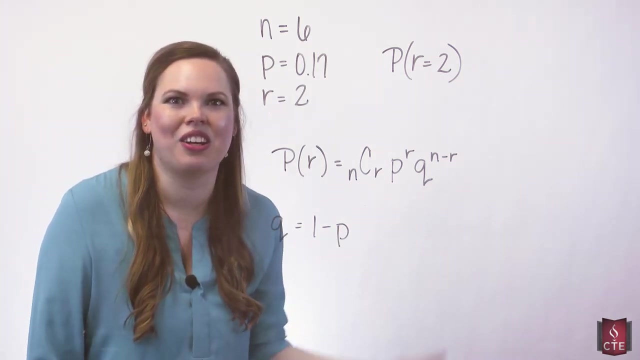 is the probability of a failure. So this is our formula. We have all of the variables except for Q, but we know that Q is the probability of a failure. So Q is 1 minus P, because P is the probability of a success, And you're going to either succeed or you're going to. 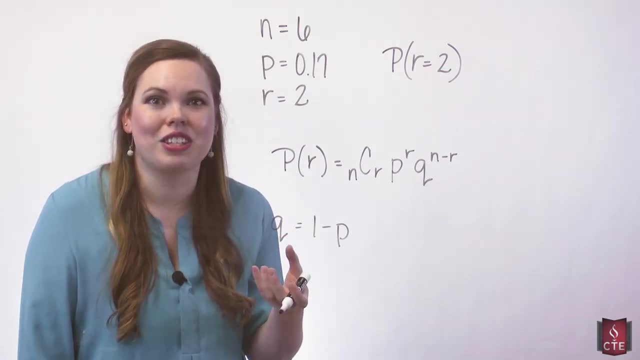 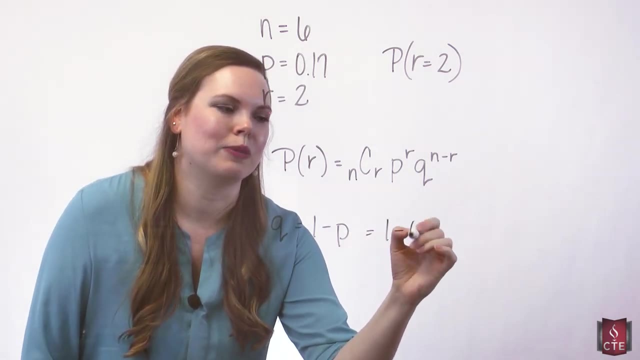 fail. So they're complements of each other. They cover the sample space, And so we know that Q is 1 minus P. They should add to 1.. So find that real quick: 1 minus 0.17 is 0.83. 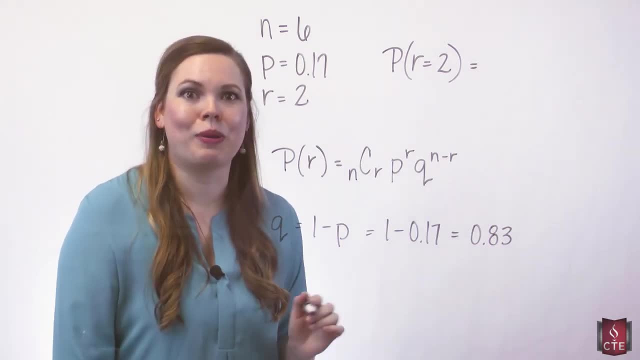 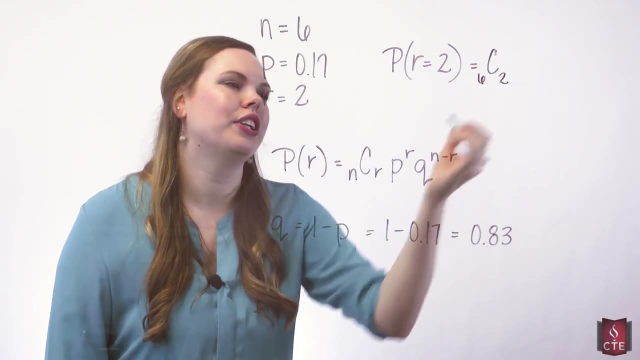 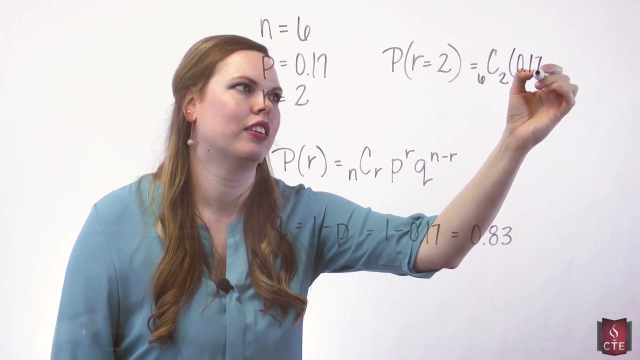 for our Q. OK, so let's just plug it into the formula. We'll start with nCr. Our n is 6.. Our r is 2.. Then we have P with probability of a success. We know it's 0.17 to the n. which is 6.. And then we have P, with probability of a success: We know it's 0.17 to the n, which is 6.. And then we have Q with probability of a success: We know it's 0.17 to the n, which is 6.. And 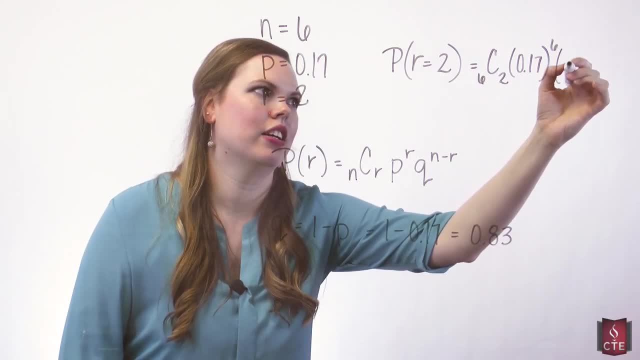 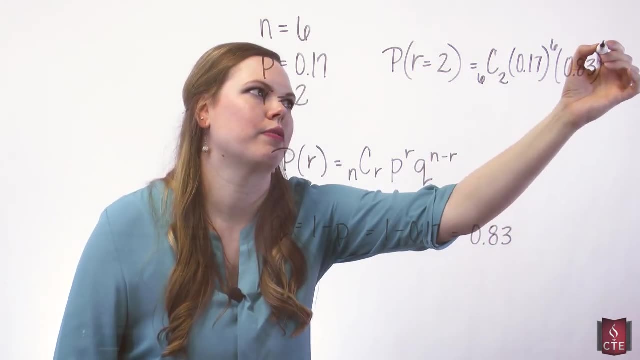 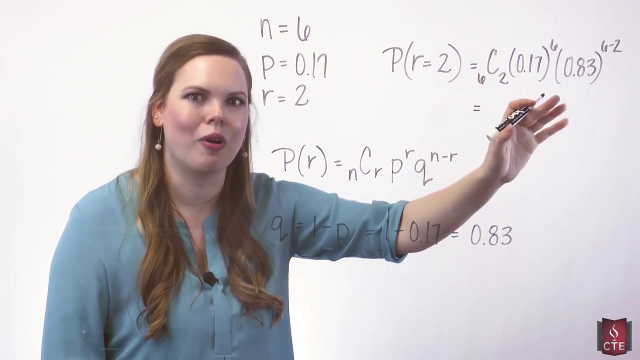 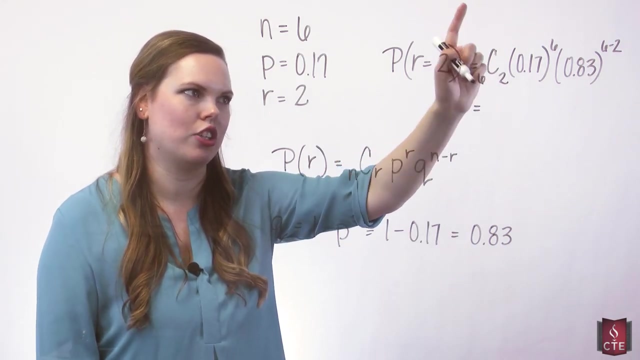 then Q, 0.83 to the n minus r, 6 minus 2.. If you do that in your calculator, calculators can handle this And you can put it all in at once so that you don't have any rounding errors. OK, so just do your combination. You could probably find your combination. write: 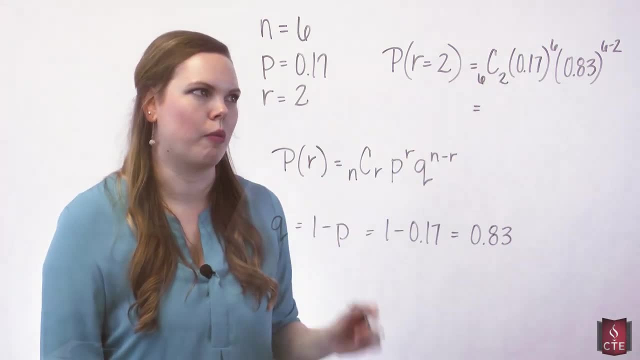 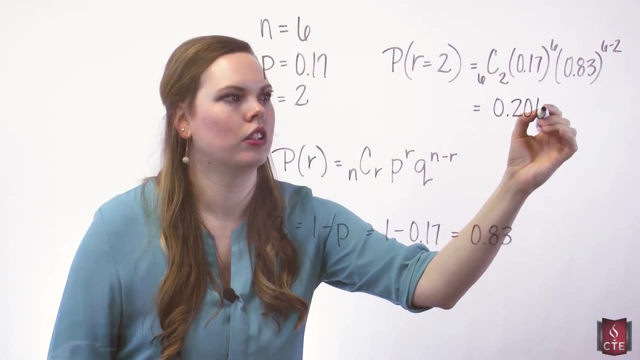 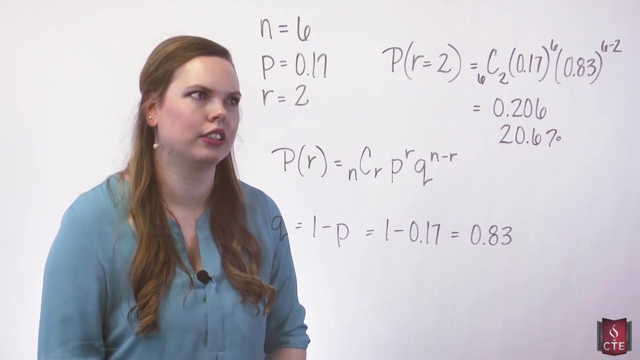 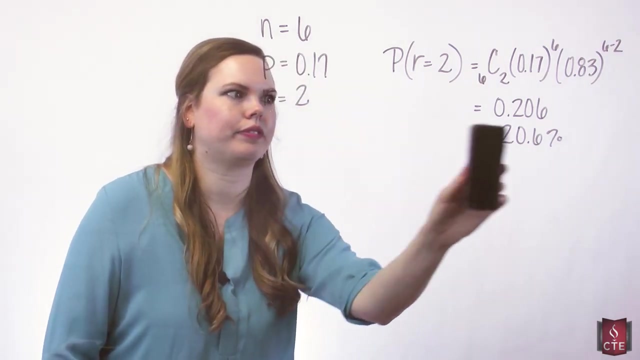 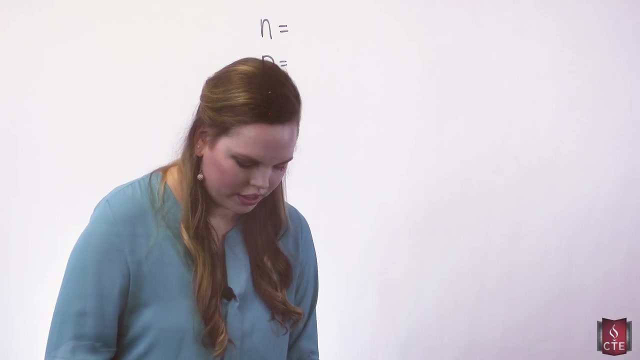 that down and then do that. times all of this at once, You should get 0.206.. So if you wanted to change that to a percentage, probability is 20.6%. Let's just quickly look at one that we could use the table for. So this is an n of 6, which is on the table.